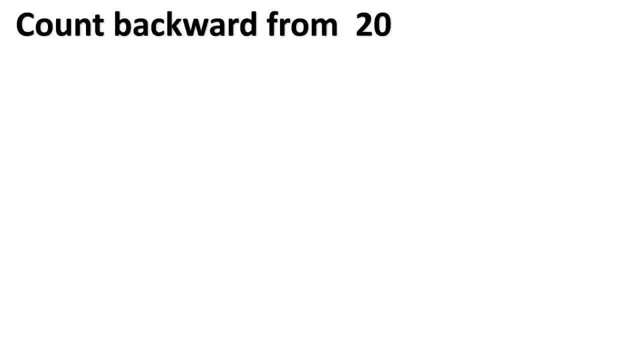 Now we're going to do count backward from 20.. 20,, 19,, 18,, 7, 16,, 15,, 14, 13,, 12, 11, 10, 9,, 8,, 7, 6,, 5, 4. 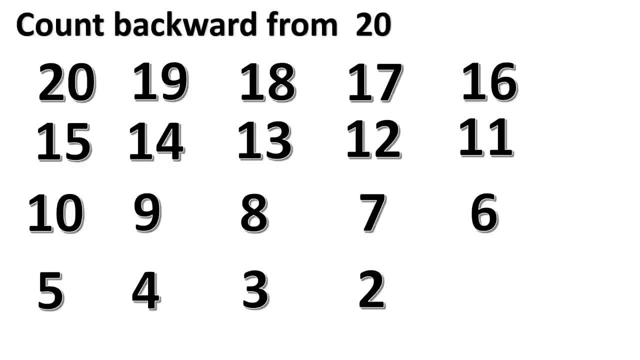 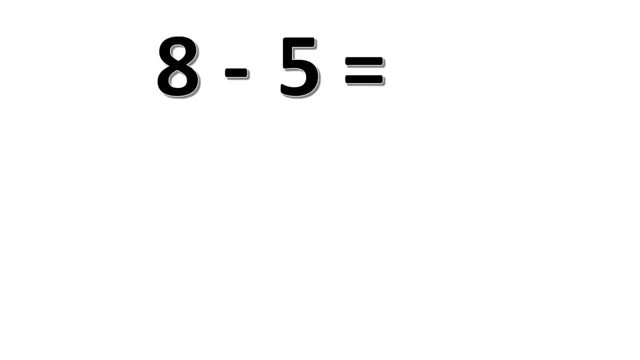 3, 2. 1 For the first example, 8 minus 5.. Which one is the bigger number, 8 or 5?? Yes, 8 is the bigger number, So we're going to start counting backward from 8.. 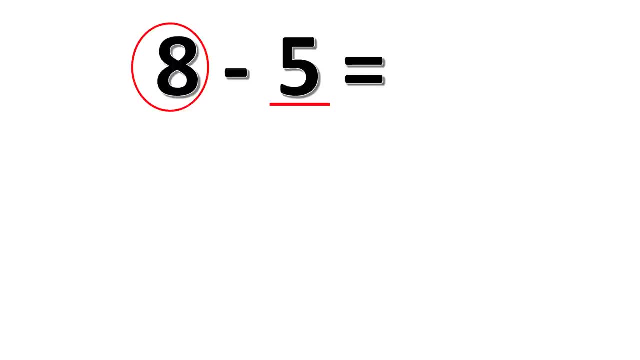 And the 5 is the smallest number. So we're going to have 5 finger ups. So, starting from 8,, 7, 6, 5., 4, 3.. So 8 minus 5 will be equal to 3.. 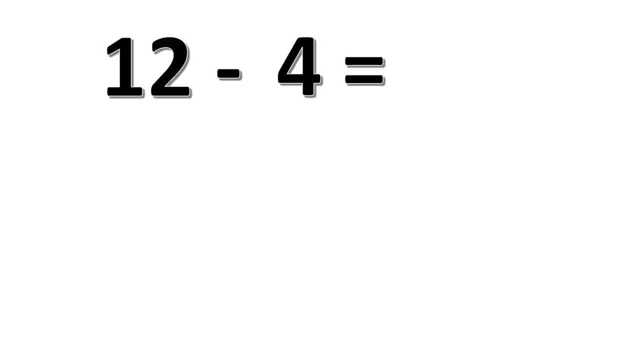 Next example: 12 minus 4.. Which one is the bigger number here? Yes, 12 is the bigger number, So we're going to start counting backward from 12.. Well, 4 is the smallest number, So let's put 4 finger up. 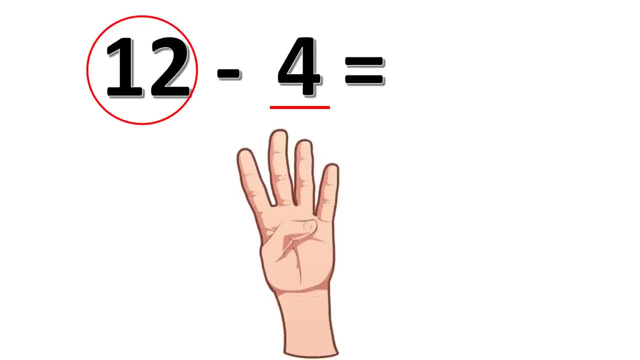 Now we're going to start counting backward from 12.. So we're going to start counting backward from 12.. So we're going to start counting backward from 12.. 12,, 11,, 10,, 9,, 8.. 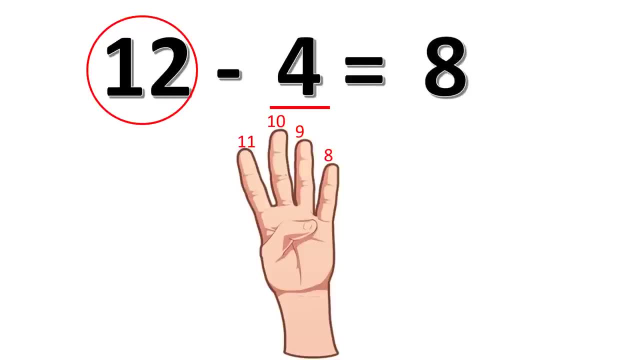 So 12 minus 4 is equal to 8.. So 12 minus 4 is equal to 8.. Kids, for the third example, we're going to solve 16 minus 7.. Kids, for the third example: we're going to solve 16 minus 7.. 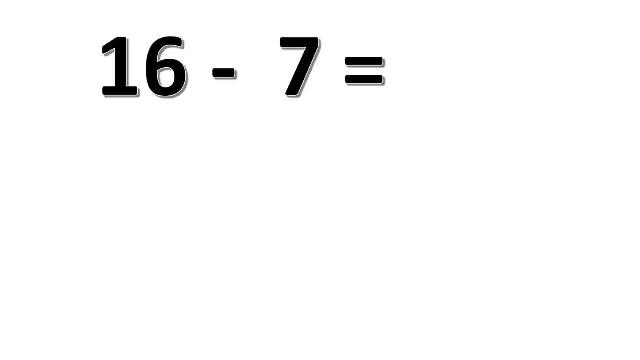 Which one is the bigger number here? Which one is the bigger number here, 16 or 7?? Yes, 16 is the bigger number. Yes, 16 is the bigger number. Yeah, we're going to start counting backward from 16.. 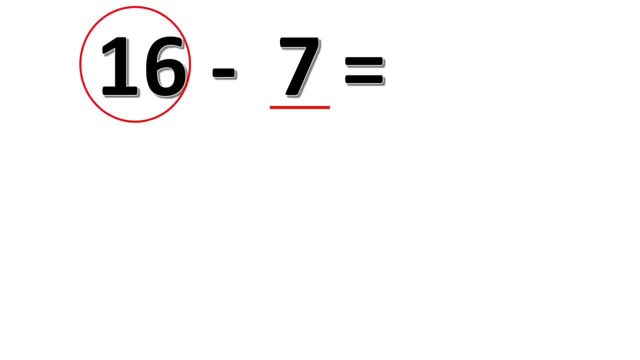 Yeah, we're going to start counting backward from 16.. And 7 is the smallest number, And 7 is the smallest number. So now let's have 7. finger up, kids. Start from 16.. We're going to count backwards. 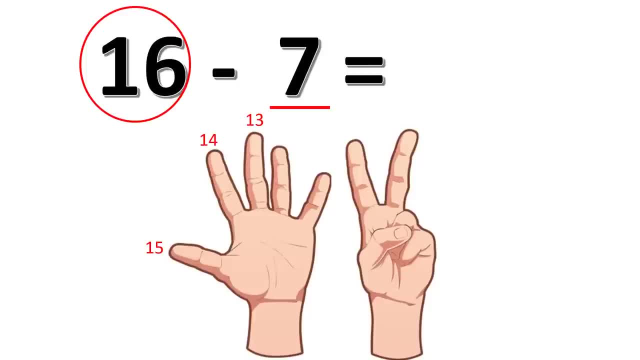 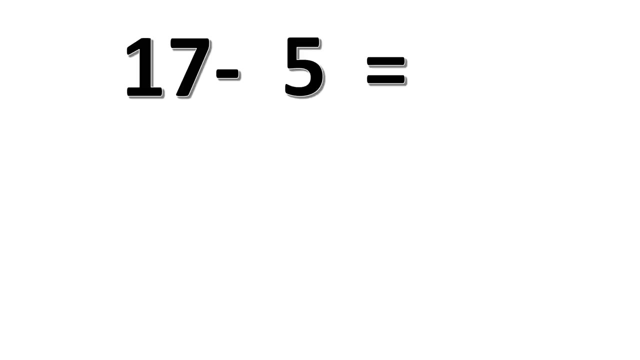 16,, 15,, 14,, 13,, 12,, 11,, 10,, 9.. 17 minus 7 is equal to 9.. Okay, kids, let's do another example: 17 minus 5.. So which one is the bigger number here? 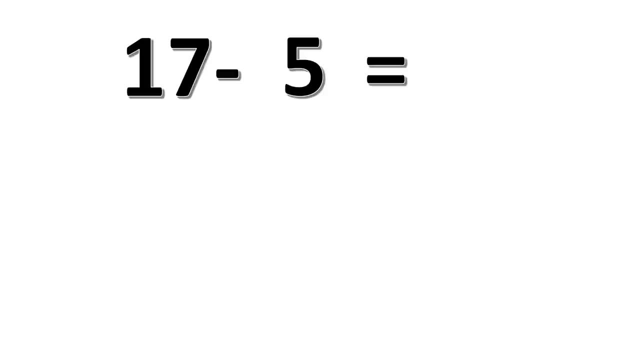 17 or 5?? Yes, 17 is the bigger number, So let's counting backward from 17.. Well, 5 is the smallest number, so let's have 5 fingers up, Start from 17,. we're going to count backward. 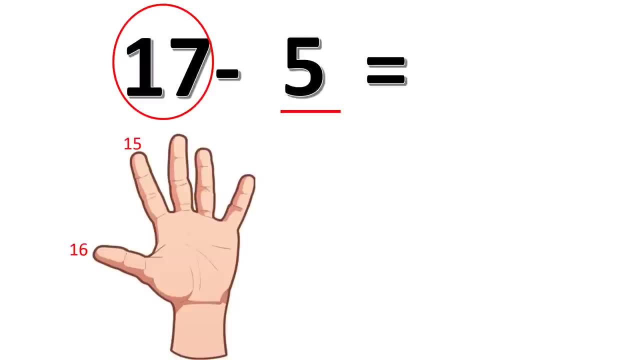 17,, 16,, 15,, 14,, 13,, 12.. So 17 minus 5 is equal to 12.. Now we're going to solve 19 minus 5.. So first, which one is the bigger number here? student. 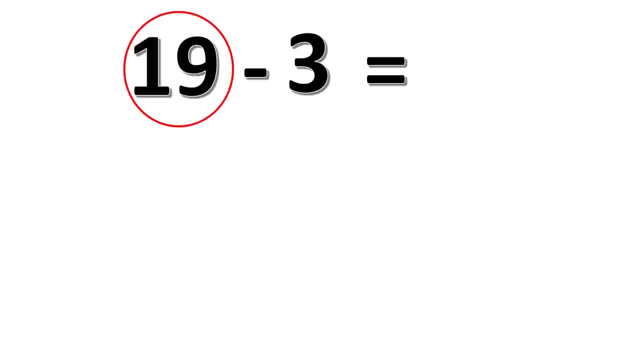 Yes, 19 is the bigger number, So we're going to start counting backward from 19.. Who is the smallest number here? Yes, 13 is the smallest number. So all of you- let's have 3 fingers up Now- start from 19,. we're going to counting backward. 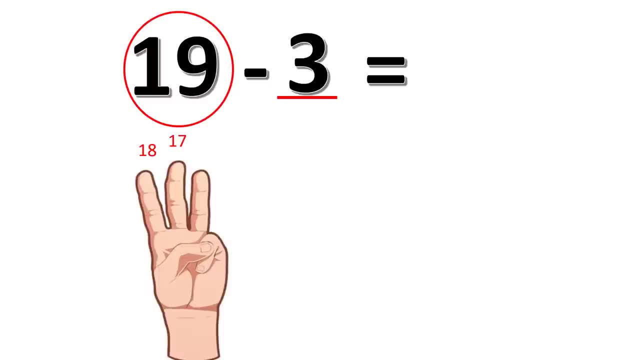 19,, 18.. 17,, 16.. So 19 minus 3 is equal to 16.. Okay, kids, we're going to do last example: 13 minus 6.. Which one is the bigger number here, 13 or 6?? 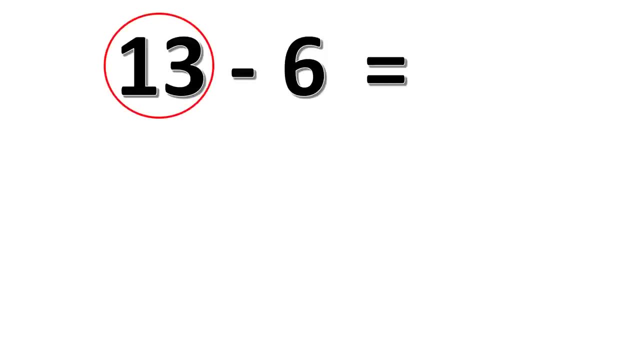 Yes, 13 is the bigger number, So we're going to start counting backward from 13.. And 6 is the smallest number. So, kids, let's have 6 fingers up, Start from 13.. We're going to count backward. 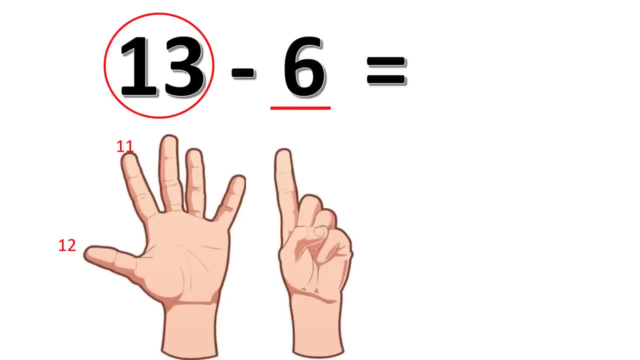